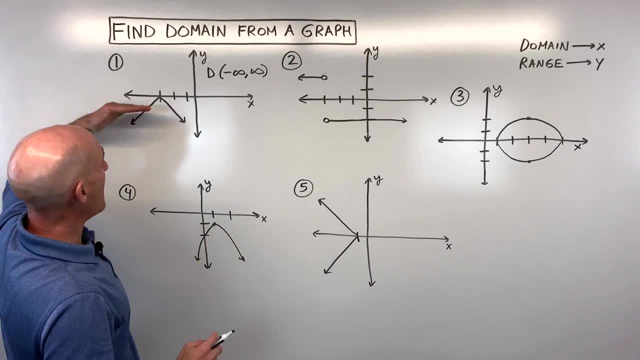 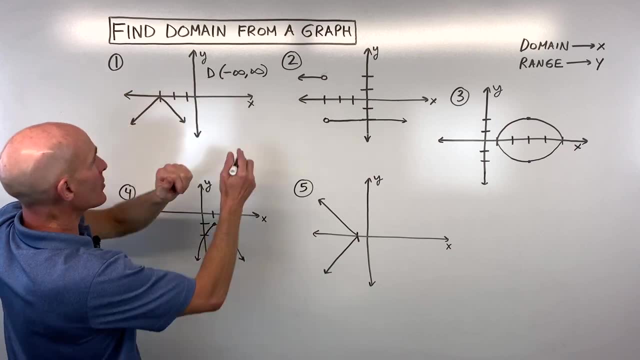 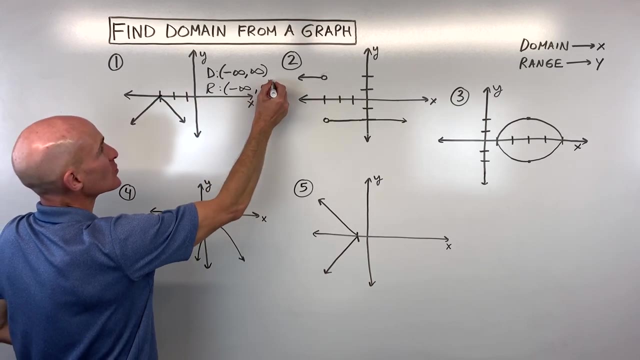 graph's going down forever and ever, But the highest it goes is right here at a y value of zero. So the range is going to be from negative infinity to zero, And it includes zero. see, it touches right here at the x-axis, So we're going to use a. 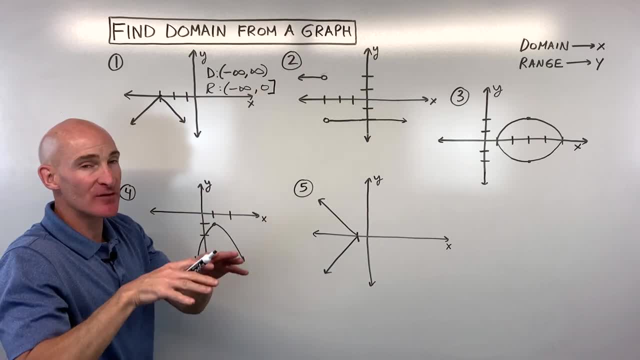 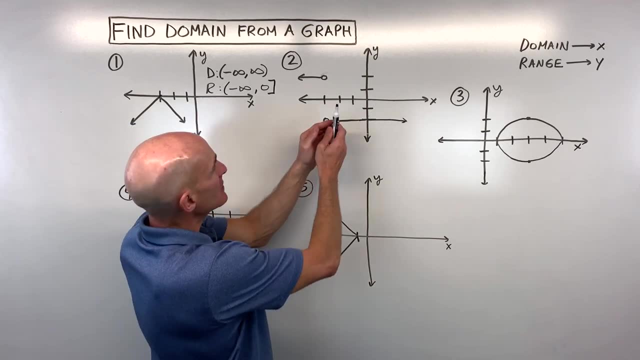 square bracket because it includes zero. Now, infinity can never reach infinity. That's always going to be like an open with the parentheses. Okay, let's look at example number two now. What do you think the domain and the range are for this one? Well, again, when I think of domain, I think 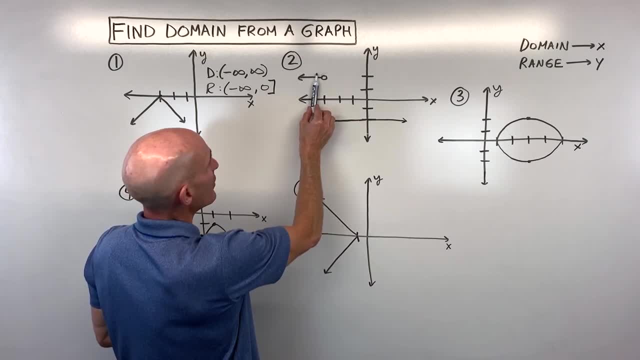 what can x be? Well, when I scan and across, see it's crossing the graph and there's a hole hole here as well. so there's basically a gap here at negative 3, let's write that down and then you can see it's crossing. 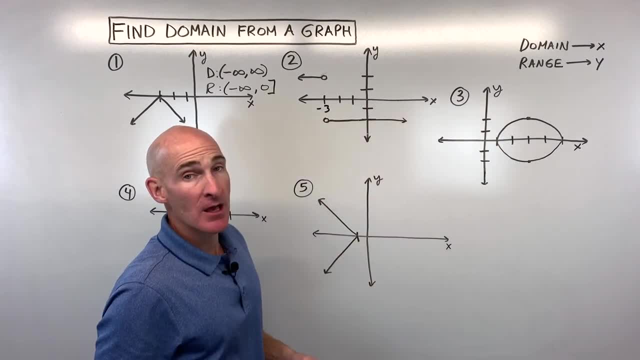 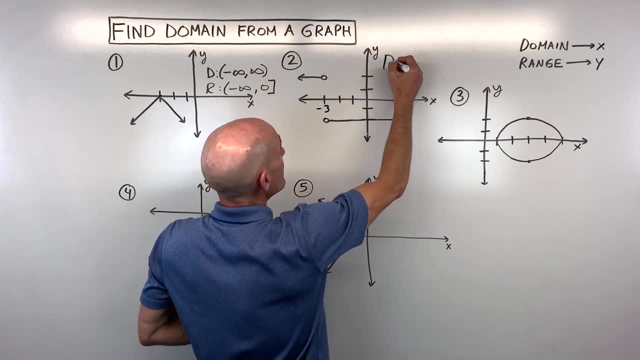 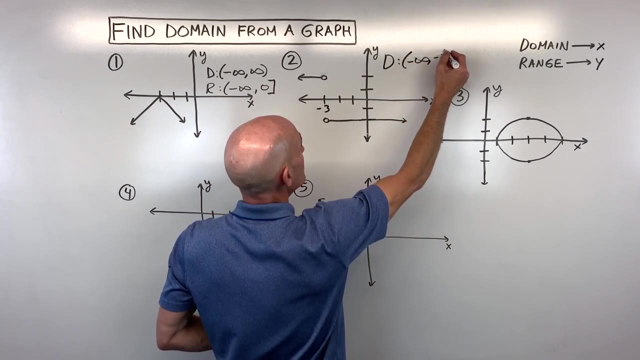 the graph and it keeps going to the right forever and ever. So essentially the domain is all real numbers except for negative 3, that's what the possible x values are. So if I was going to write this I would go from left to right. so that's negative infinity to negative 3, not including 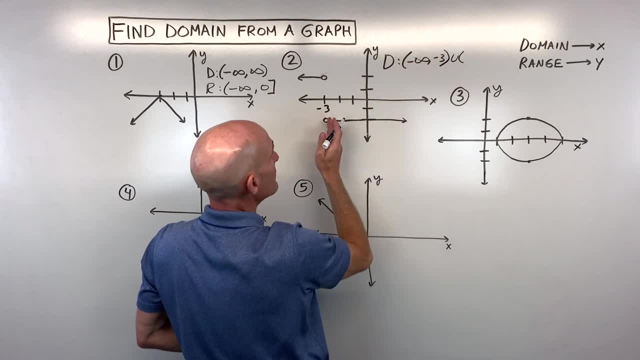 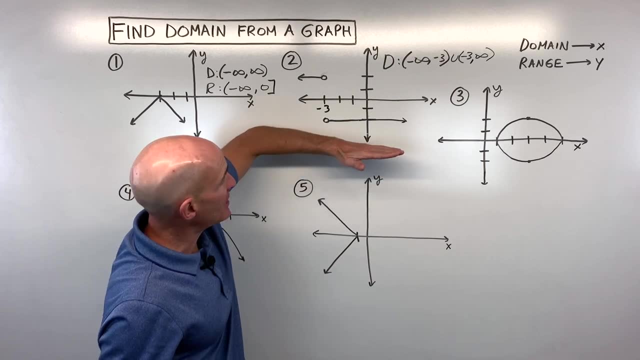 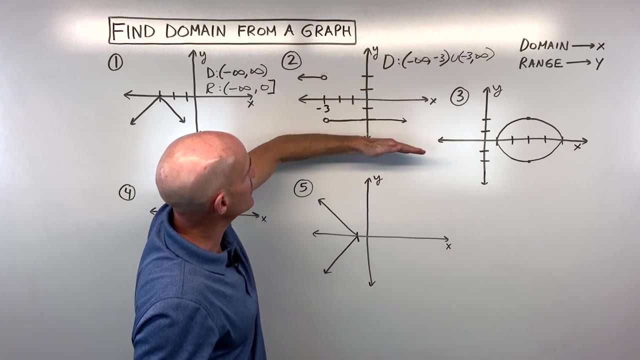 negative 3, so we use the parentheses and then it picks up at negative 3,, not including negative 3, all the way to positive infinity. Now, if I was going to do the range, these are the y values. so I take a horizontal line, like my forearm here, and I go from low to high and it looks like 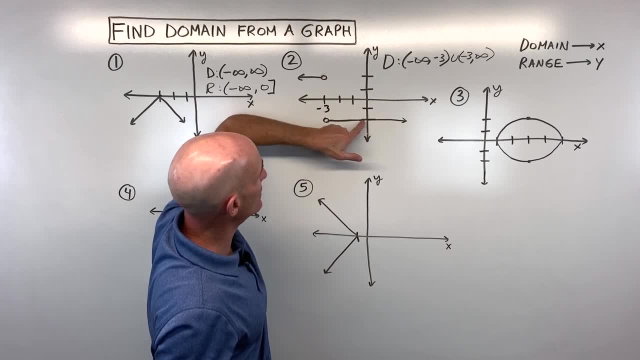 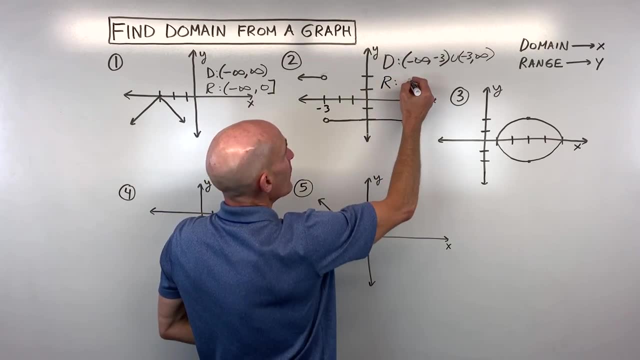 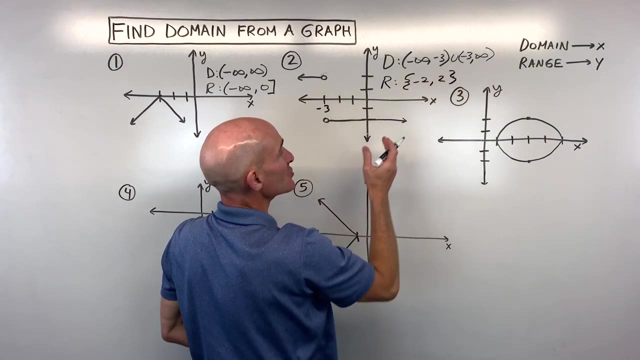 because these are horizontal lines, the y values can only be here at negative 2, and then it jumps to positive 2, and it's really just those two numbers. So instead of writing an interval, I would just use this set Bracket notation. I would say negative 2 and positive 2, and just draw those curly Q set. 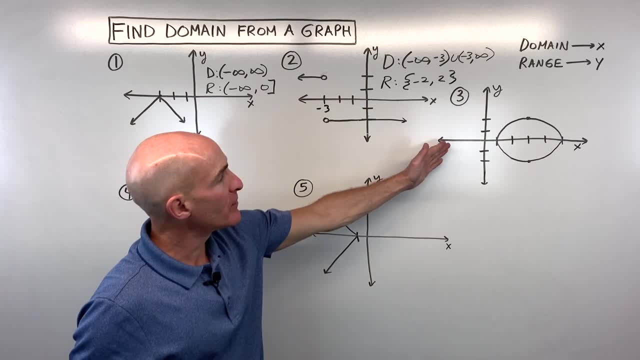 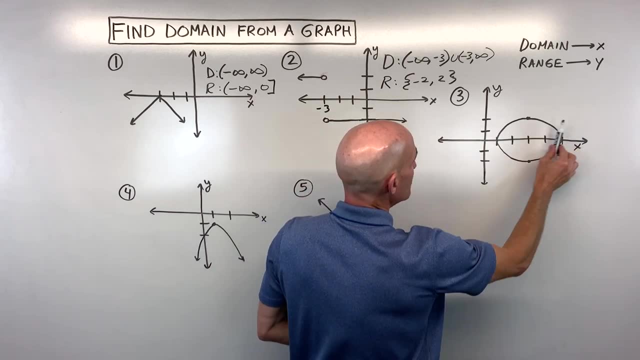 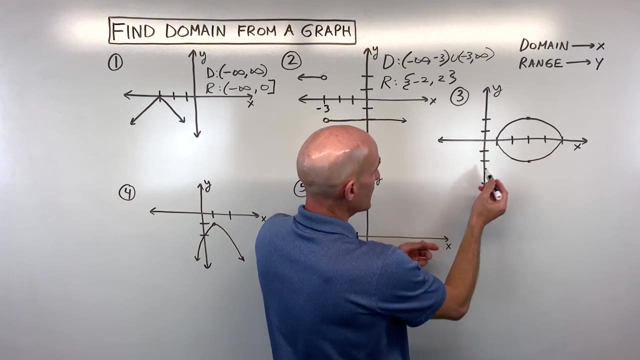 brackets. okay, so those are the only y values. What do you think for number 3, domain and range for this one? Hmm, well, the domain again. what can x be Scanning from left to right looks like from 1 to 5, and it includes 1 and it includes 5, so I would say domain is 1 to 5,. 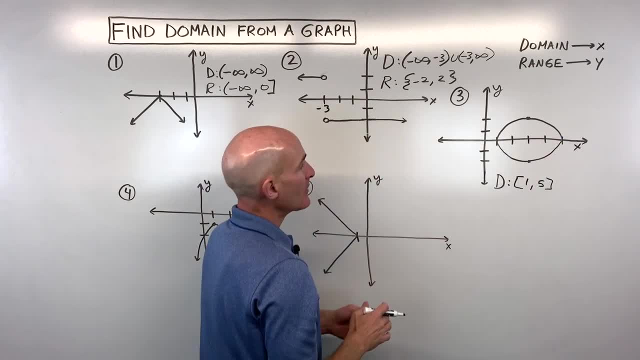 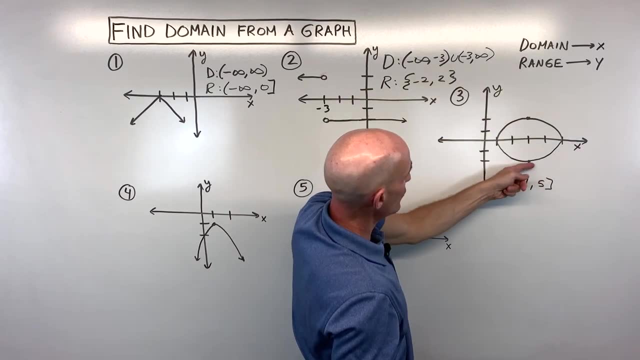 using the square brackets because it includes those values and then the range. what can the y values be? See, low to high. see, I'm going in the y direction, which is like the vertical direction. the lowest it can be is negative 2,. it includes all these values here up to positive 2,. 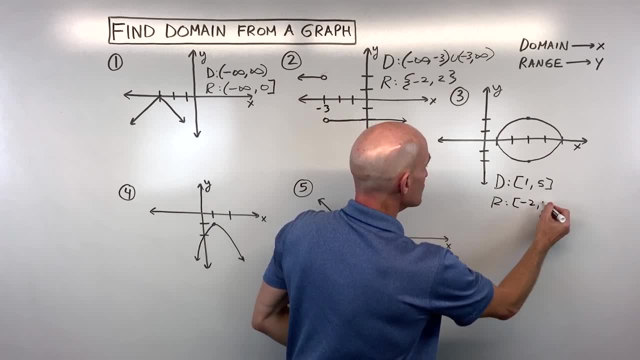 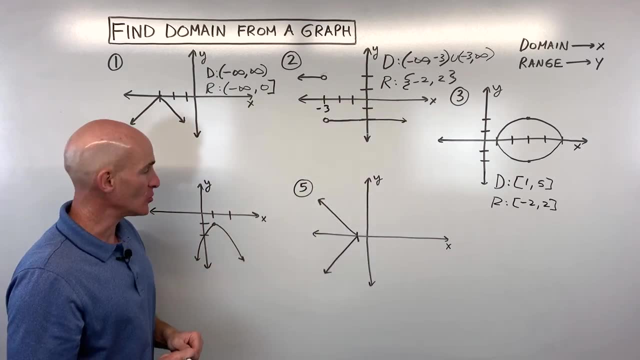 so I would say a range is negative 2 to positive 2, inclusive. Okay, and then what do you think for 4 and 5? Maybe pause the video and try these two for practice. So for number 4, what can the 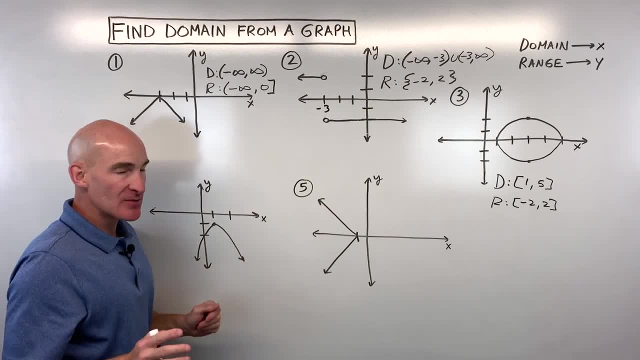 be? What can the x values be? Now, sometimes people get a little bit confused by this one, because you see how this is like a parabola. It's kind of like a U-shaped graph. Sometimes students will say: well Mario, how do you know? this graph doesn't eventually like become? 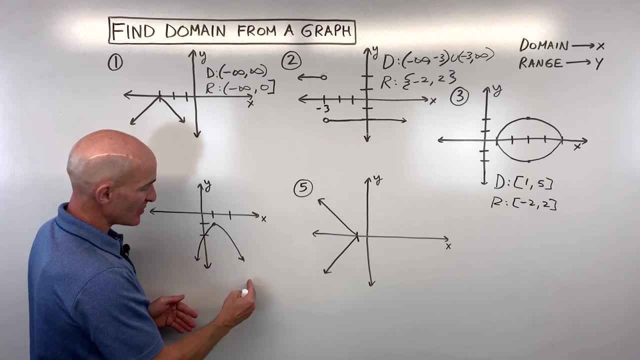 like a vertical line, Like it's curving, It's getting like steeper and steeper. in a sense, How do you know? it doesn't just go vertical. Well, with these it's going to gradually go to the left and the right, forever and ever. So in this case, the domain is going to be: 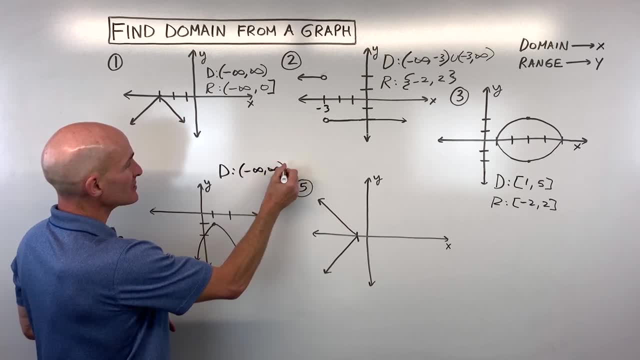 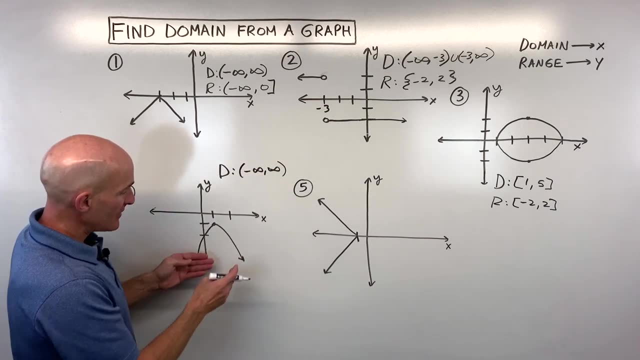 all real numbers, or we could say negative infinity to positive infinity, Whereas the range going from low to high, okay, looking at our y values, our vertical direction, this goes down to negative infinity and it goes all the way up to this negative one. So here, 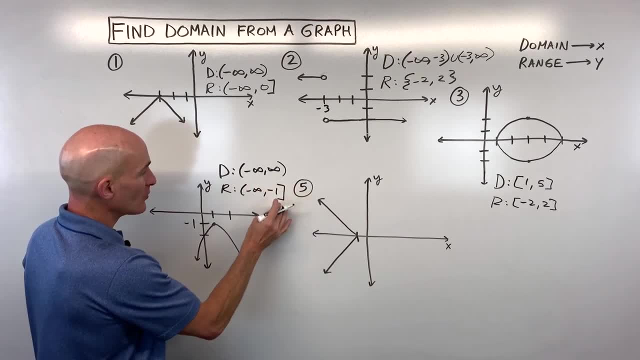 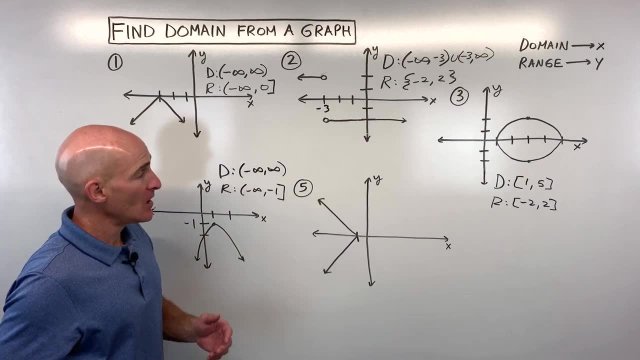 we'll say the range is negative, infinity to negative one. We're using the square bracket of negative one because it includes negative one. Infinity, remember, is always open. You can't really reach infinity. And then for number five, what do you think? 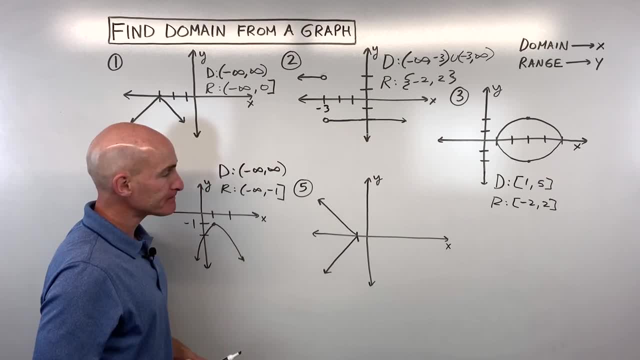 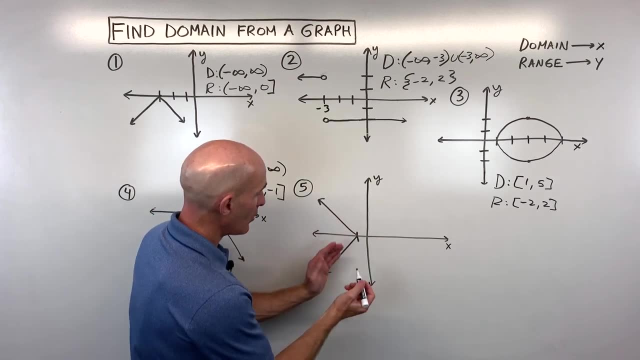 For this one, what did you get for the domain and the range? Well, for this one, again for domain, I think. about what can x values be? It's going to be from negative infinity all the way to negative one. So let's write that down: Negative infinity to negative one. 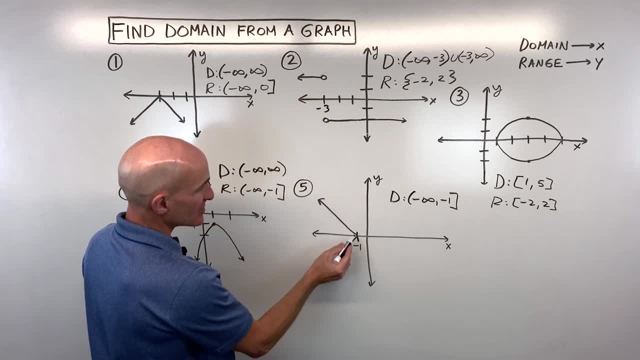 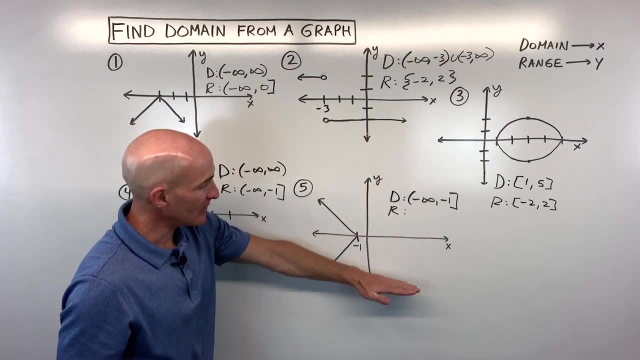 including negative one. See how it touches negative one. It's not an open circle, That's closed. And then the range. what can the y values be? We can go from low to high. We're thinking of the vertical direction, Down, down, down forever. So negative infinity. this is going up, up, up forever And it hits.